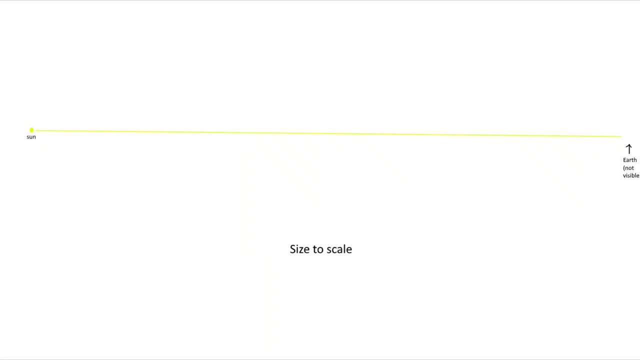 The earth is so far and small that the rays of the sun hit it essentially in parallel. But forget about that for a sec. So here's an ology bomb for you. Earth spins. Now here's a second ology bomb. Earth is a sphere, so earth is essentially a spinning ball. 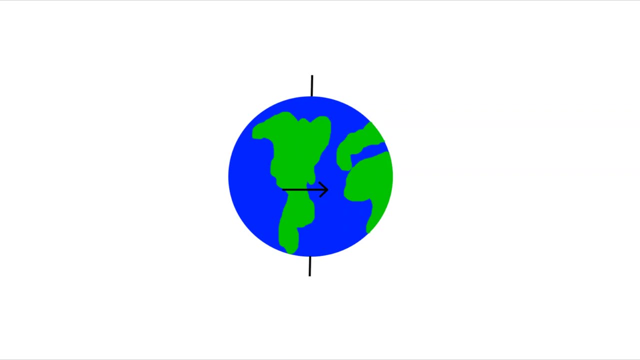 Now, as it comes with spinning balls, you get two poles, The poles in a spinning ball, of course, being the exact two points which don't move, Two spots completely opposite of each other. They do not rotate On earth. we call them the north pole and the south pole. 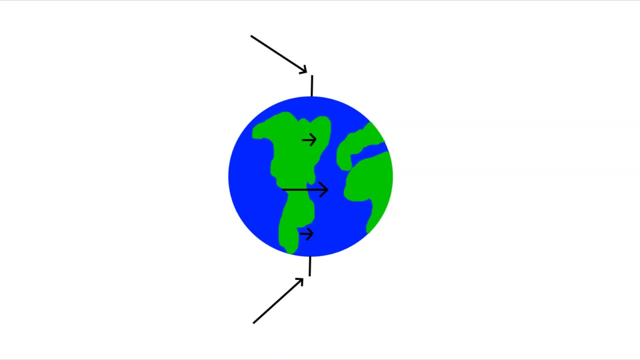 North and south being completely arbitrary directions, as space does not have an up or down Great. But we can go further. Exactly in between the two poles, we have an imaginary line which rotates the fastest. you can say Splitting the spinning ball into two halves, Two hemispheres if you like. 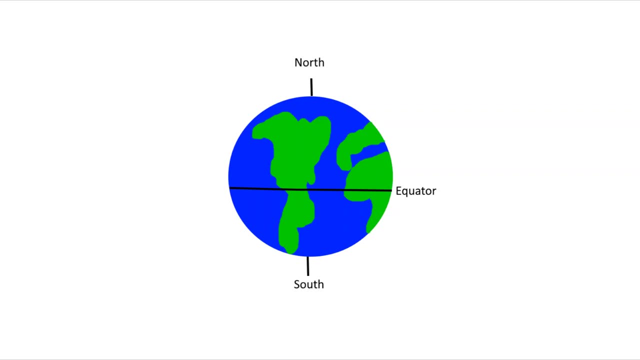 This line is, of course, the equator. Everything north of the equator is in the northern hemisphere, And the south of the equator is in the southern hemisphere. Now here's where numbers, unfortunately, come in. We can name a point on earth using coordinates: latitude and longitude. 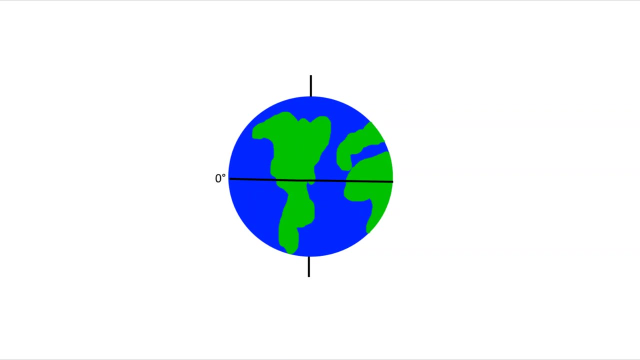 This is what latitude is, Because the poles are exactly opposite of each other and the equator is exactly in between the two. we can name them and everything in between them using angles. Now imagine that the equator is zero degrees. 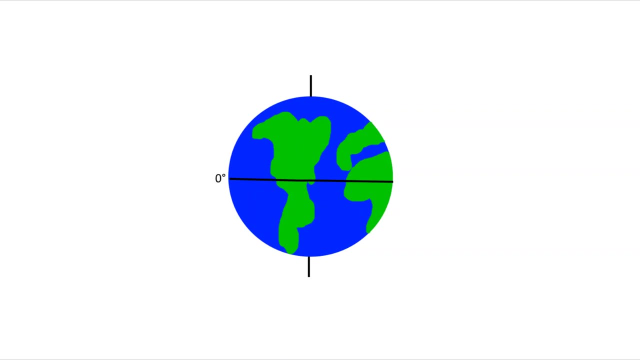 The north pole is, of course, 90 degrees away from it, while the south pole is of course also 90 degrees away in the opposite direction. So 90 degrees north and 90 degrees south. Let's go in between the equator and the north pole. 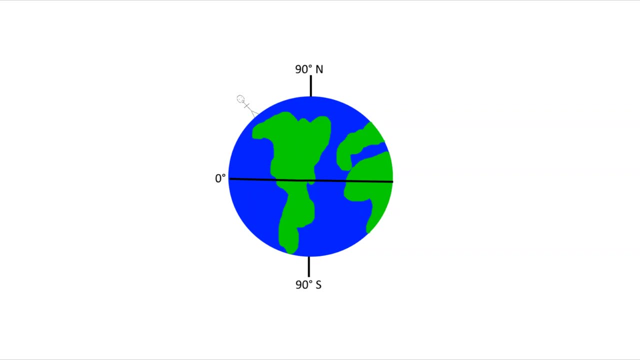 Suppose I stand there in between them. What's my latitude? 45.. 45 north to be specific, to differentiate between the two hemispheres. Notice how the 45th latitude, or alternatively the 45th parallel, is 45 degrees away from the equator and the north pole. 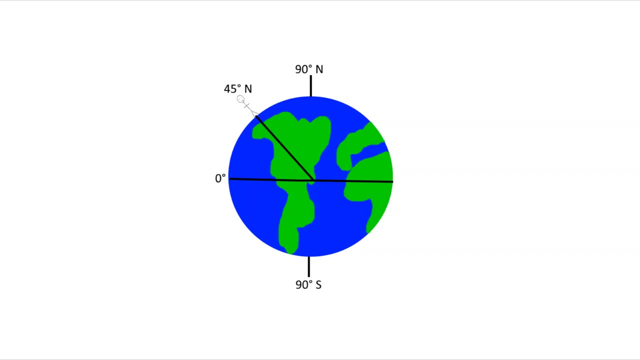 Imagine a line going from the equator and the 45th parallel to the center of the earth. where they will meet. The angle between them will be 45 degrees. That's latitude. Now I'm on vacation in Uganda And I visit the equator, and it's noon.